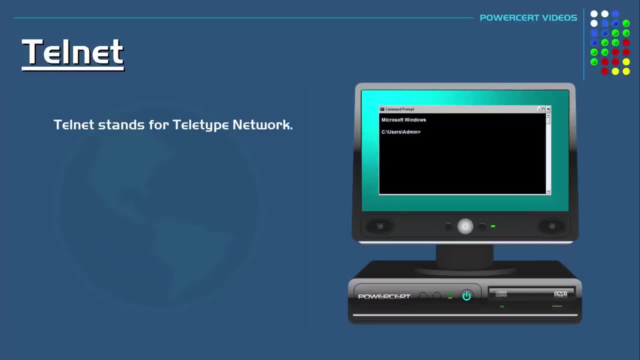 fast Now. Telnet stands for Teletype Network and it was developed back in 1969. And because it was developed prior to the internet, security was not really an issue. So with Telnet all the commands are sent and cleared, So you can use it to run a computer. you can just use a simple dumb terminal. 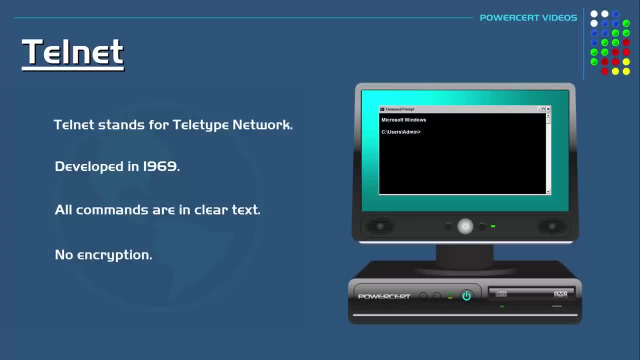 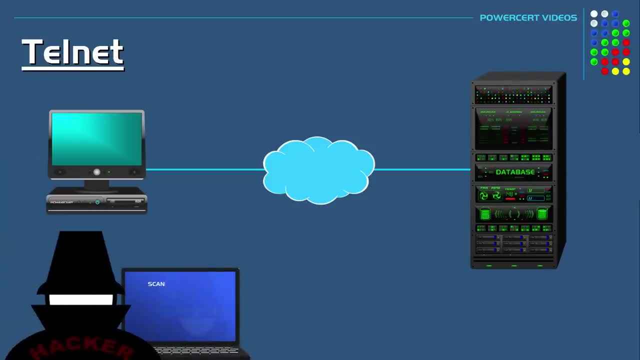 and all the commands are sent and cleared. So if you were to use Telnet today to communicate with a server over the internet, someone could easily eavesdrop and grab any sensitive data that you're sending to that server, such as usernames and passwords. So, because of the lack of encryption, 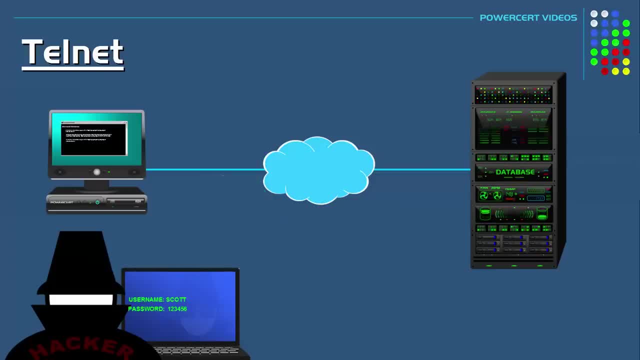 Telnet is outdated and it should not be used over the public internet. But some people still use it today, but largely in a local area network and not over the internet. But also they may have to use it if they are working with older equipment that can't support. 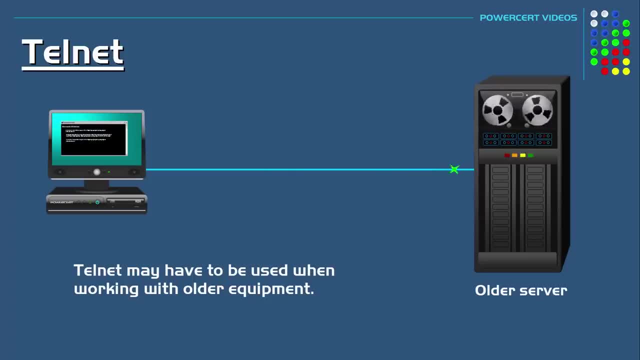 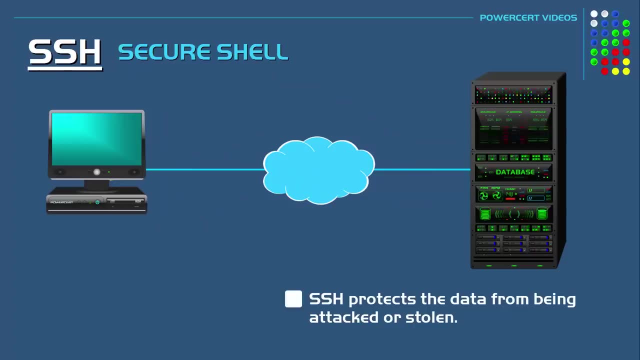 modern protocols such as SSH. Now, SSH or Secure Shell is a better alternative to Telnet. Secure Shell protects the data from being attacked or stolen as it's being transferred over a network. So, as I stated before, if you are sending sensitive data like a login or password, 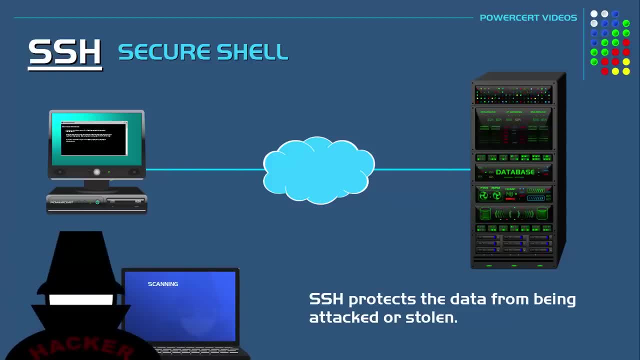 a hacker could be listening and steal the data. Now, this is the reason for Secure Shell. Secure Shell encrypts the data during the transfer and protects it from potential threats, And in addition to encryption, it also provides password and public key authentication. So Secure Shell does everything that Telnet does. 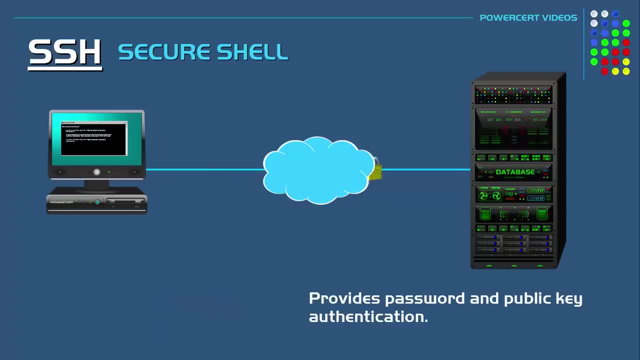 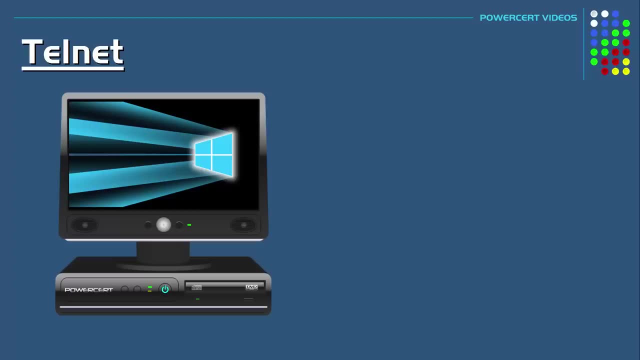 but it's a secure protocol And that's what people use today instead of Telnet. Now, if you want to see some interesting examples of Telnet, you can do this on your computer, And in my example, we're going to do this on a Windows machine. 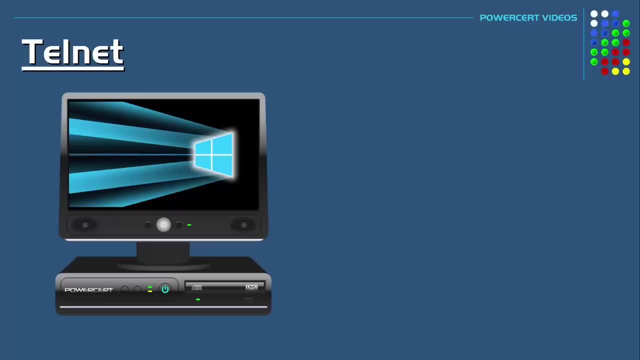 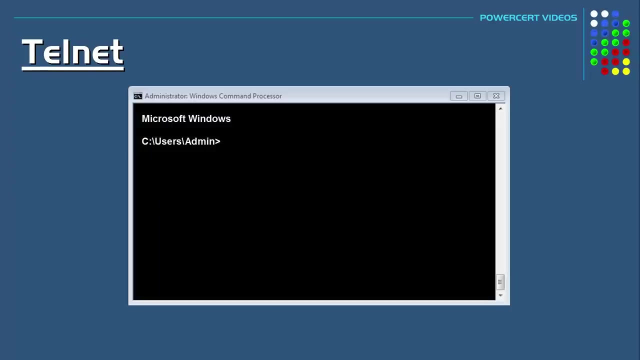 Now, first you have to enable the Telnet client in the Windows operating systems. So you first go into programs and features and then you would click on turn Windows features on or off, And from here you have to enable the Telnet client feature, And then you would just open up a command.